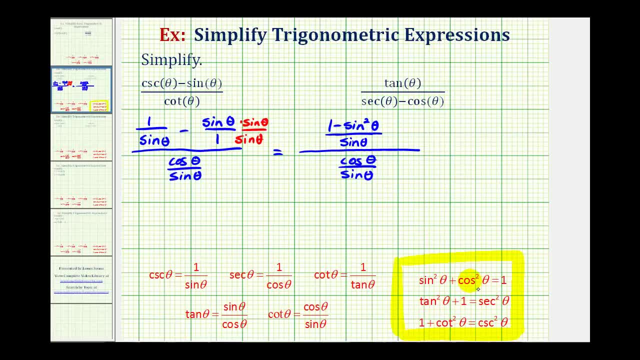 If we subtracted sine squared theta on both sides, we would have cosine squared theta equals one minus sine squared theta, So we can substitute Cosine squared theta for one minus sine squared theta. So this would give us cosine squared theta all over sine theta. 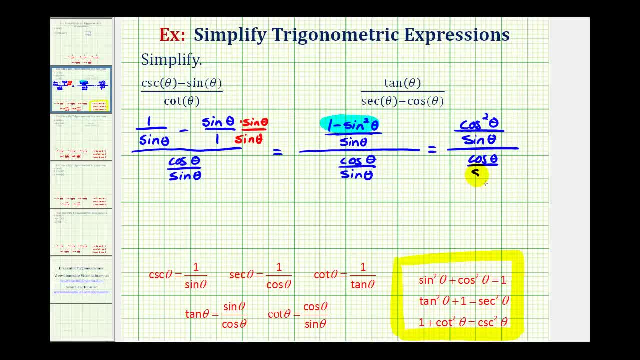 And then we still have cosine theta over sine theta in the denominator. Now remember: a fraction bar means division, So let's go ahead and write this as a division problem. We would have cosine squared theta over sine theta, divided by cosine theta over sine theta. 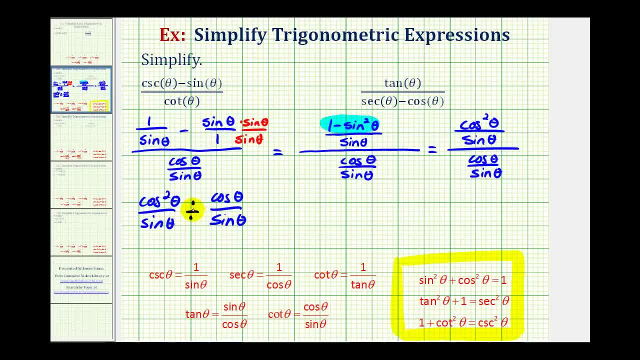 But every division problem can be written as a multiplication problem if instead of dividing by this fraction here you multiply by the reciprocal, or in this case multiply by sine theta over cosine theta. So this would give us cosine squared theta over sine theta. 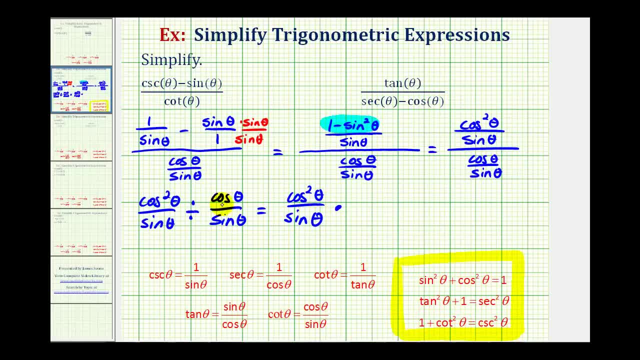 Notice how the first fraction stays, the same times the reciprocal of the second fraction. So it's sine theta over cosine, theta over cosine theta. and finally we can start to see some factors that will simplify. Here we have sine theta over sine theta and notice that here we have two factors. 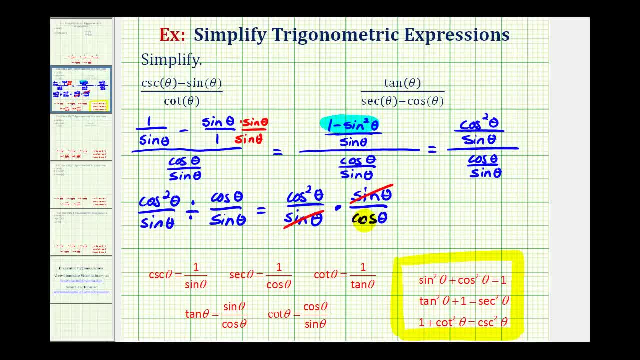 of cosine theta. here we have one factor of cosine theta. So one factor of cosine theta simplifies out, leaving us with one factor of cosine theta. So the given expression simplifies to cosine theta. Let's take a look at the second expression on the next slide. 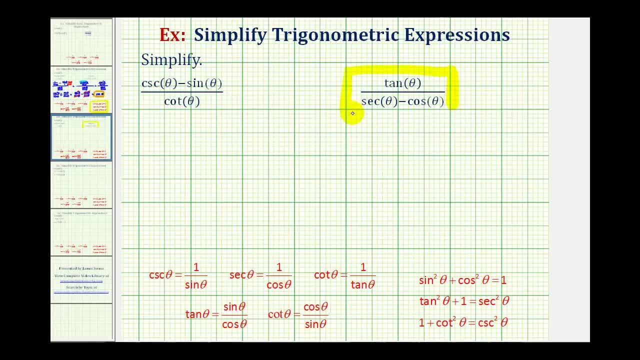 So again, now we're going to simplify this expression. Notice, one of the trig functions are squared, so we'll go ahead and convert everything to sine and cosine again and see where that leads us. Well, tangent theta is equal to sine theta divided by cosine theta. and then 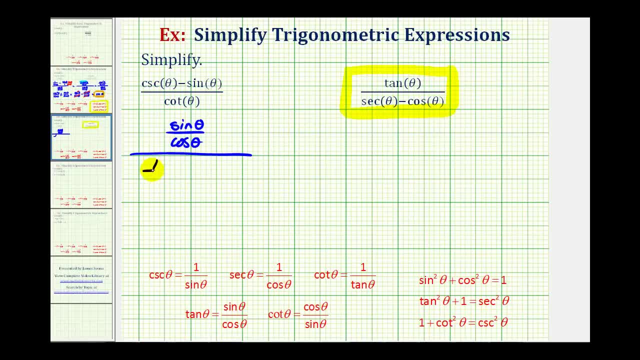 for the denominator secant theta is equal to one over cosine theta, and then for cosine theta, because this is in fraction form, we'll write this as cosine theta over one. So, just like in the previous example, the only thing that we can possibly do is subtract these. 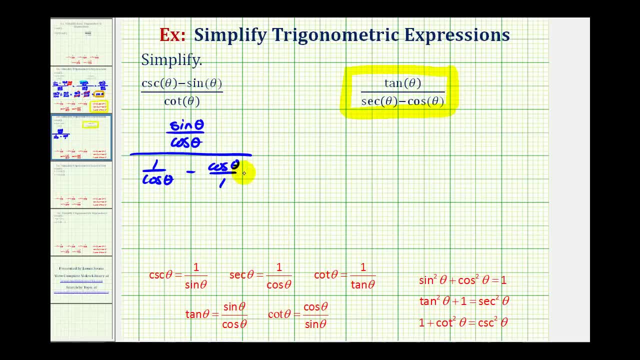 fractions here by obtaining a common denominator which now would be cosine theta. Now we're going to multiply this by cosine theta over cosine theta, So for the moment the numerator is going to stay the same and then, on the bottom, notice how the common denominator is now cosine theta. 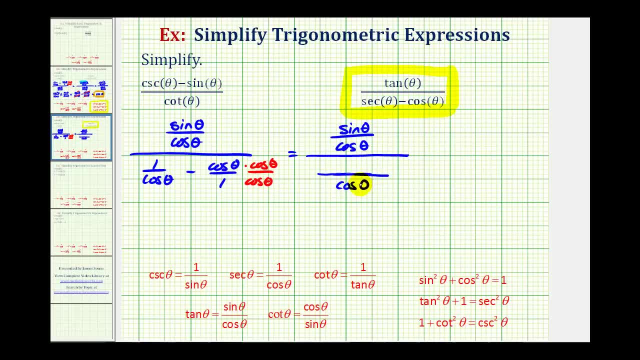 So we sum this up here: theta and the numerator would now be one minus cosine squared theta. Now, notice, we have a trig function squared, or in this case one minus cosine squared theta, which should lead us to this identity here. Notice, this time if we subtract cosine. 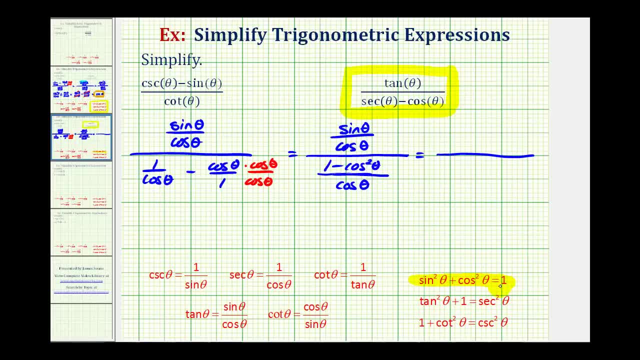 squared on both sides, we would have sine squared theta equals one minus cosine squared theta. So we can substitute sine squared theta for one minus cosine squared theta. So our denominator is now sine squared theta over cosine theta. Now let's see if we can skip the division problem and write this as a multiplication. 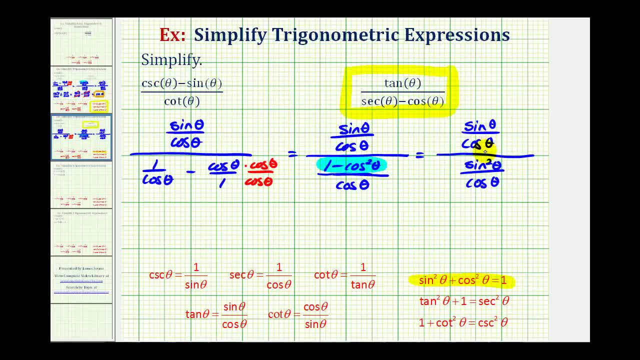 problem Right now. this is sine theta over cosine theta, divided by sine squared theta over cosine theta, which means, as a multiplication problem, the first fraction stays the same, And then, instead of dividing by this fraction here we're going to multiply by the reciprocal. So it's going to be times cosine theta over sine squared theta, And 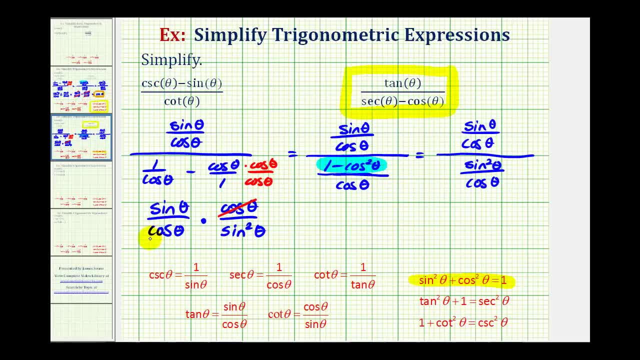 now we can see this is going to simplify nicely. Cosine theta over cosine theta simplifies to one, And here we have two factors of sine theta. Here we have one factor of sine theta. So one factor will simplify to one. This will simplify to one. This will simplify to one factor of sine theta, So we have one over. 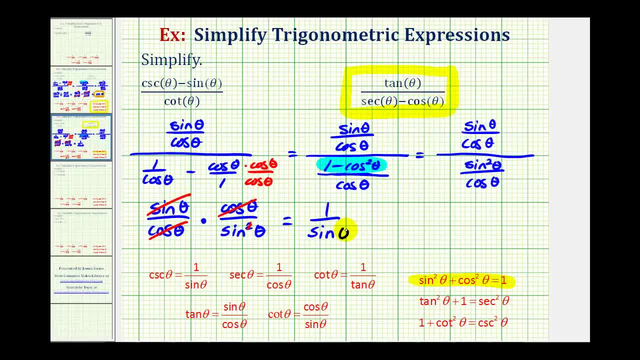 sine theta. So we do have it in terms of one trig function, but it's still in fraction form, And since one divided by sine theta is equal to cosecant theta, we'll go ahead and write this as cosecant theta, So the given expression. 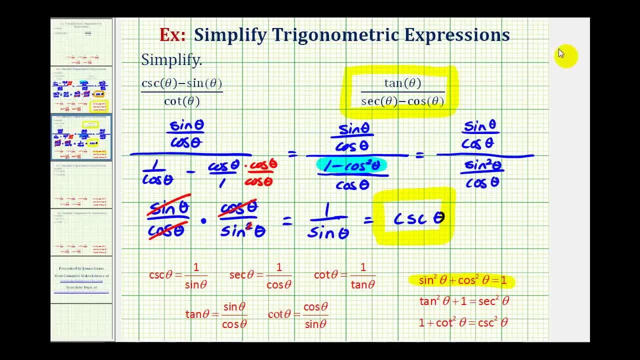 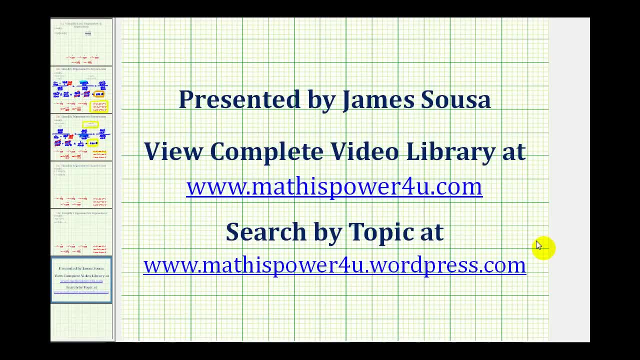 simplifies to cosecant theta. I hope you found this helpful. We'll look at some more examples in the next few videos.